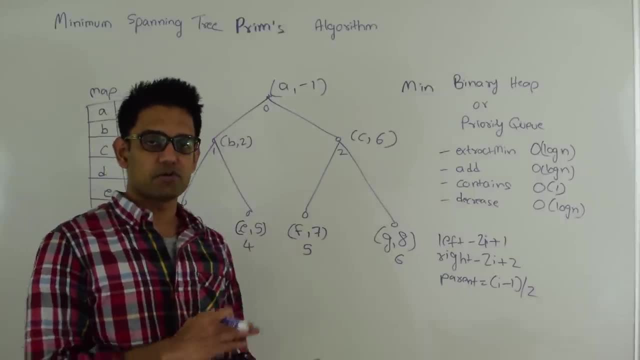 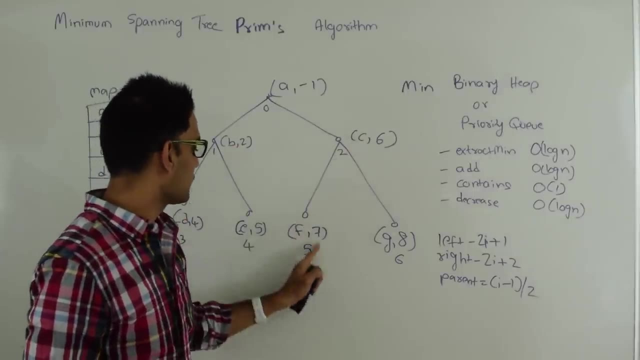 that value at every node is less than or equal to both its children. So minus 1 is less than or equal to 2 and 6, 2 is less than or equal to 4 and 5, 6 is less than or equal to 7. 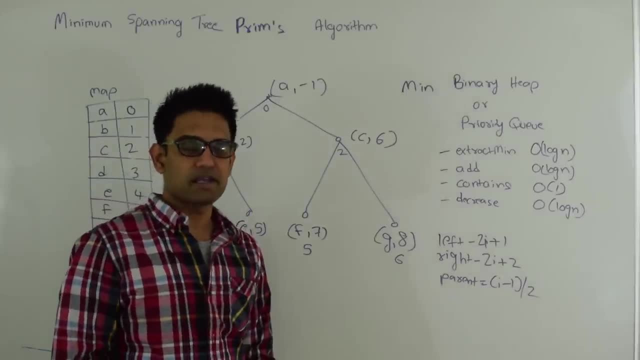 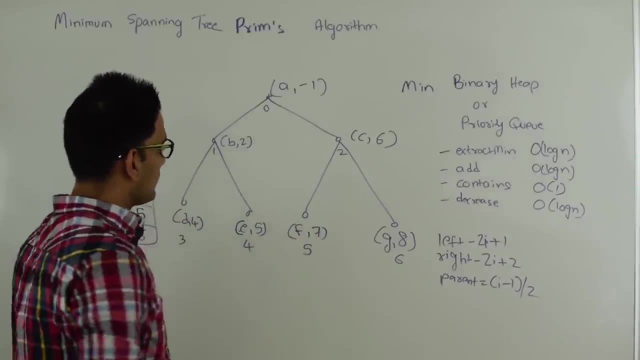 and 8.. So this satisfies all the properties of minimum binary heap. Also, we know that values of the minimum binary heap are stored in array, So this is just a logical diagram. In reality, this pair is stored at location 0,. this pair is stored at: 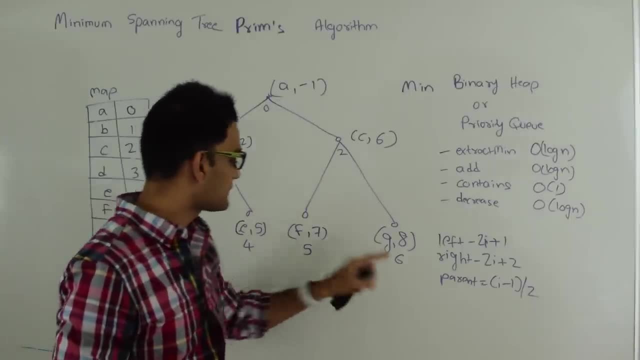 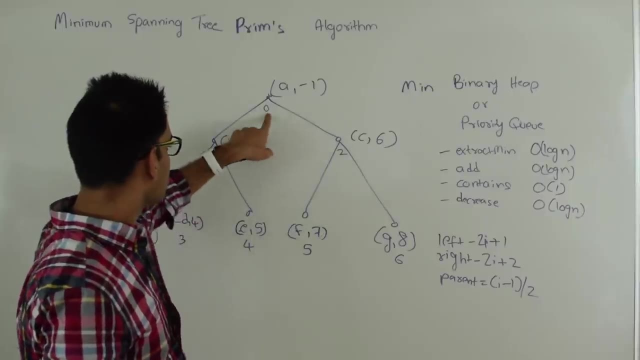 location 1, location 2, location 3,, 4,, 5 and 6 of array. To get the left child we apply this formula: 2i plus 1.. So to get this guy's left child in the array we replace 0 with i, So 2 into 0 plus 1. 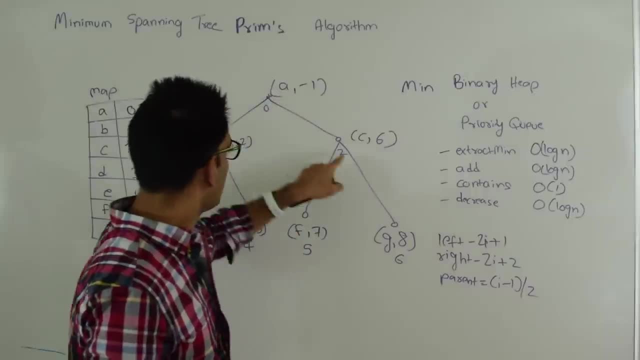 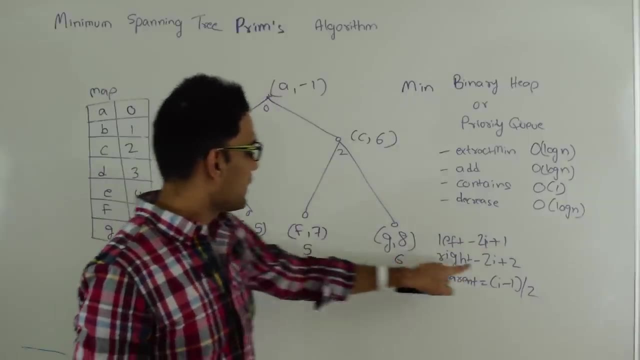 so that's 1.. So this is left child and 2 into 0 plus 2.. So this is right child. For 2's left child, we replace i with 2.. So 2 into 2 plus 1. So that's 5 and. 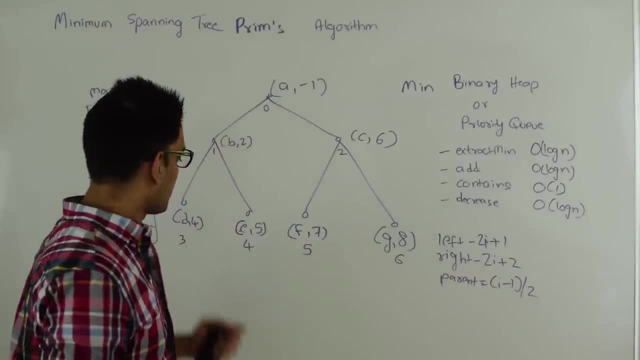 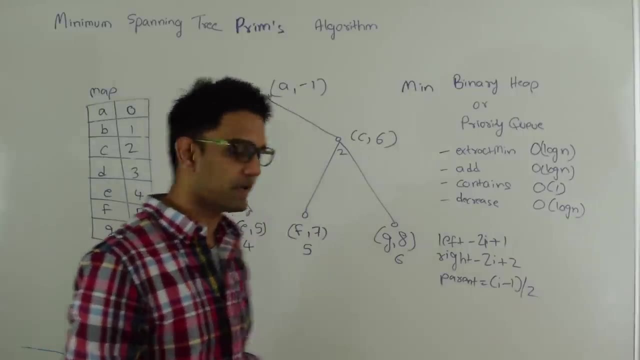 2 into 2 plus 2.. So that's 6.. So that's its right child. And to get a parent, for example to get 4's parent in array, we replace 4 with i, So 4 minus 1, 3 by 2, so that's 1.. So 4's parent is 1.. So this is. 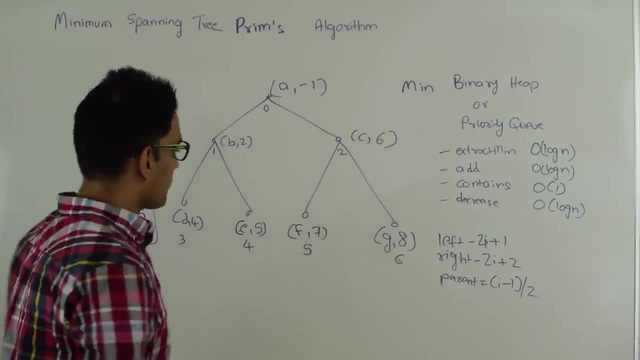 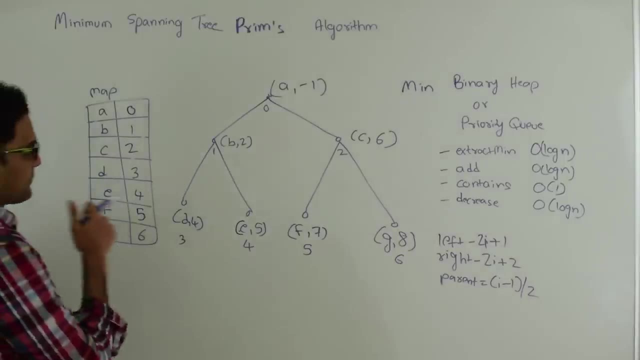 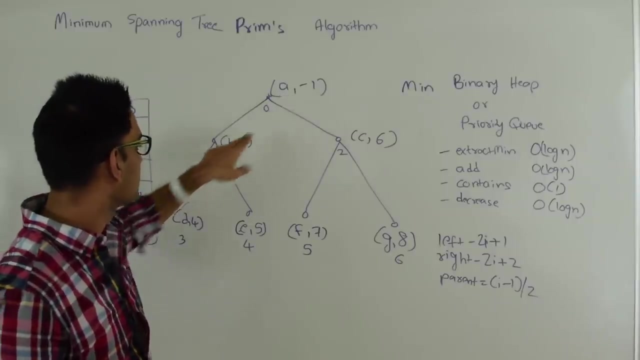 how regular binary heap works. Now, to support these two contains and decrease operation, we need another map. We need another data section map to do that efficiently And in this map we are going to store this key, So every pair here is identified by this key. unique value key. 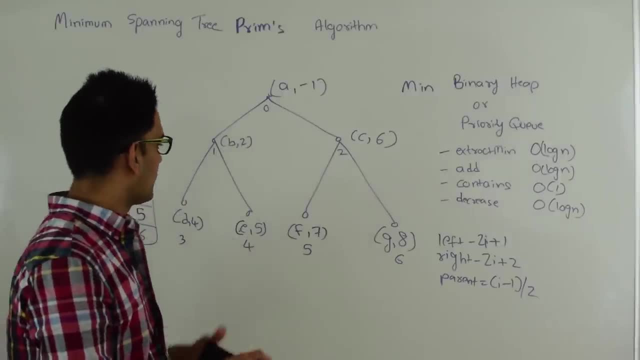 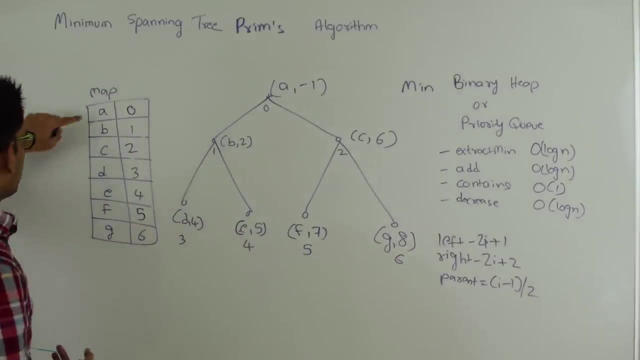 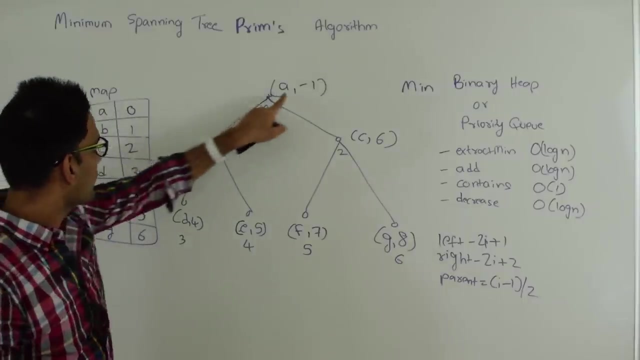 And the second value here is just used to position them in this binary heap. So now to check. so the way this map works is the key here. is this key and the value here is the position in the array. So a is stored at location 0, b is stored at location 1, c is stored at location 2 of array. 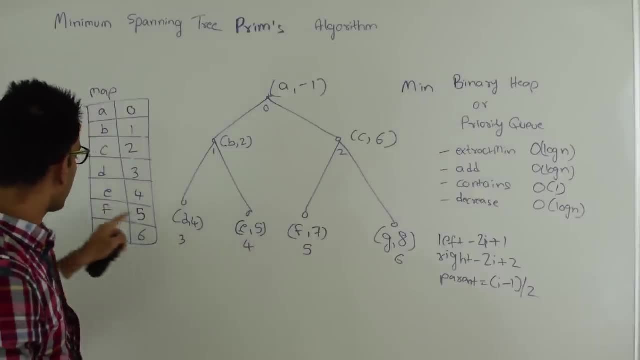 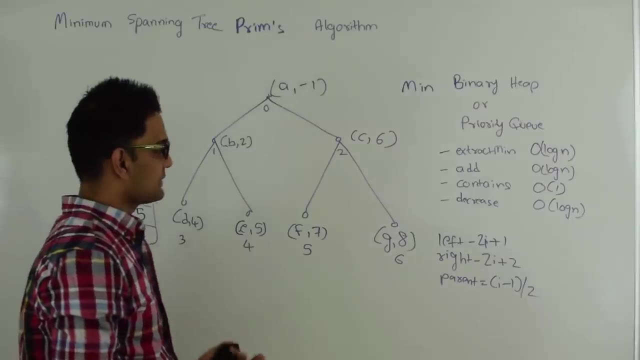 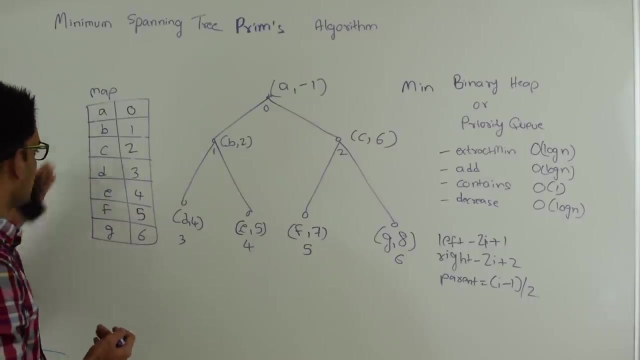 d is stored at location 3, e at 4, f at 5 and g at 6.. So now to support contains operation. what we do is we check: does this heap contains c? So all you have to do is go to this map and check: does this map have a key c? and yes, it does. So this can be done. 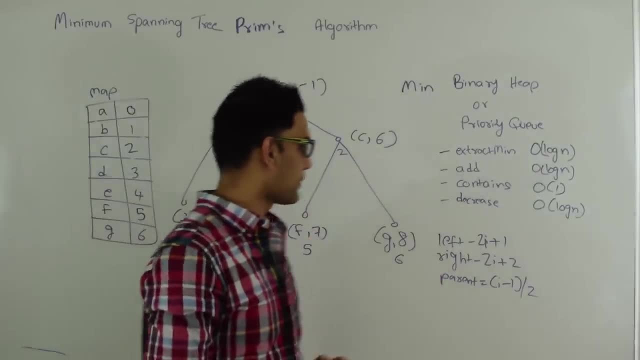 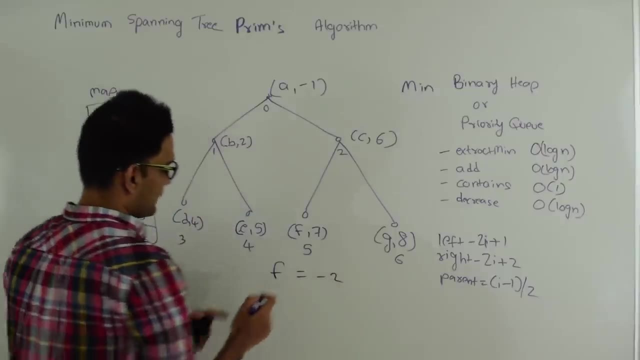 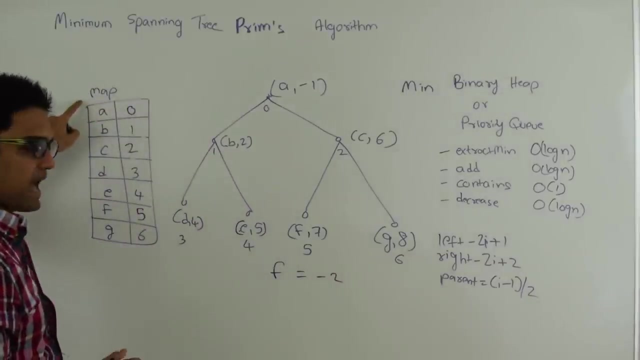 in a map in O of one time. What about decrease operation? So let's say we have to decrease the value of 5 to minus 2.. So decrease this 5 to minus 2, this f to minus 2.. So what we do is we first come to this map, check where. 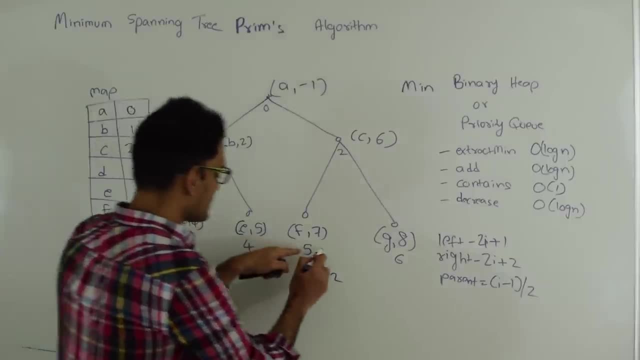 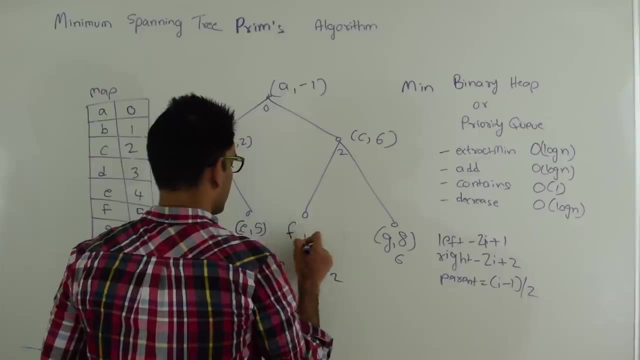 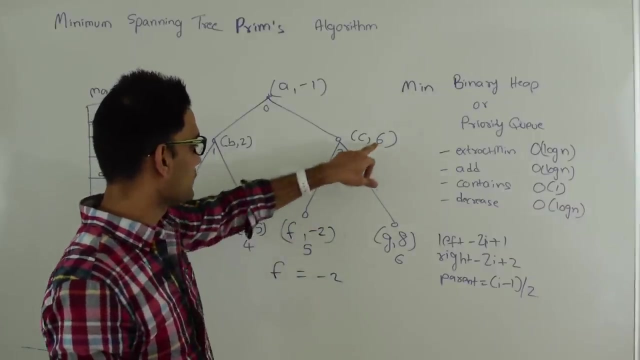 this f is stored, So f is stored at location 5, so we reach this point. Now we change the value here to be f and minus 2.. At this point it violates the property of binary heap- minimum binary heap- because this value is less than its parent. So, using this, 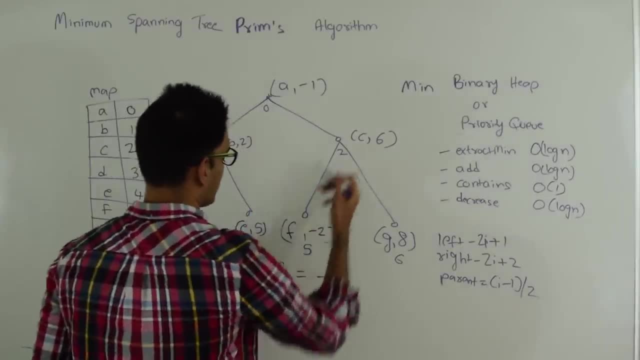 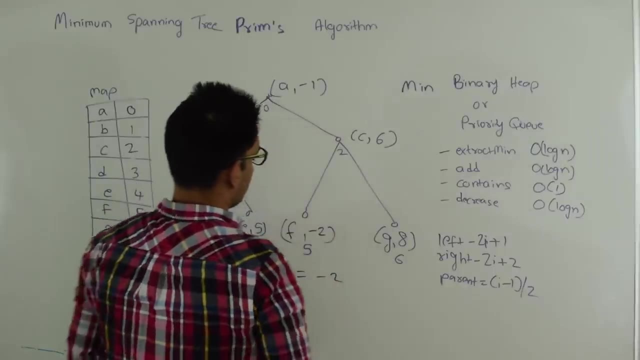 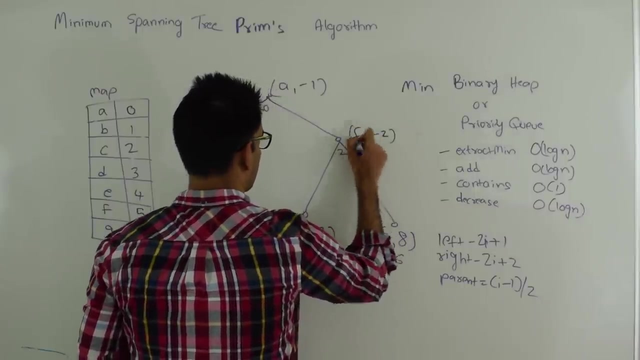 formula: i minus 1 by 2, so 5 minus 1 by 2, so that's 2.. We check if this value is less than this. It is, So we are going to swap this data here. So here we get f minus 2, and here we have c: 6 and. 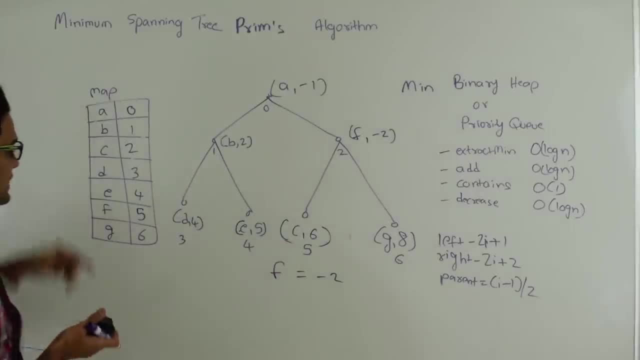 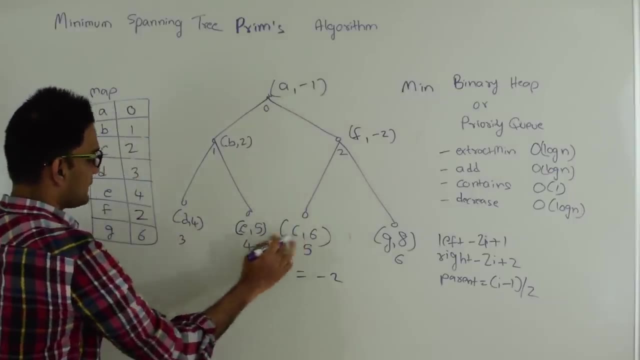 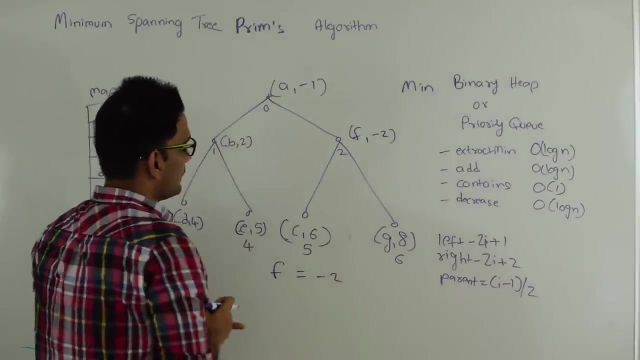 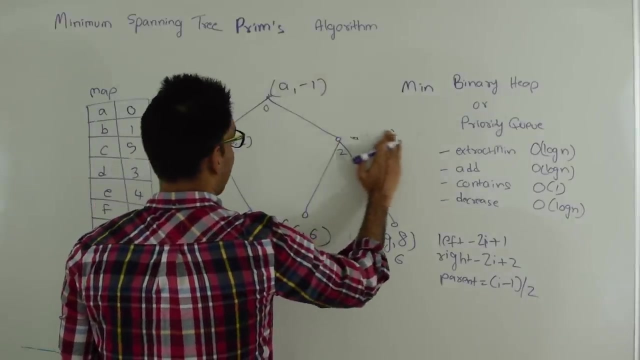 also we have to go into this corresponding map and change their locations. So f's new location is 2 and c's new location is 5.. Now this f is still violating this property here, because minus 2 is less than minus 1.. So again, we are going to do a swap here. So a minus 1 is here and 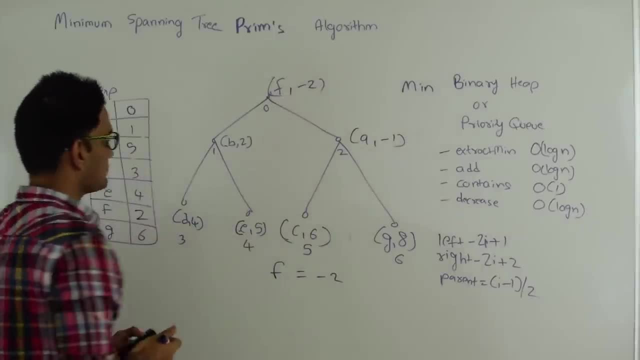 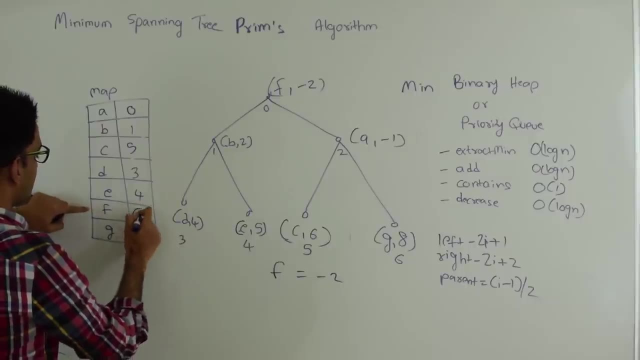 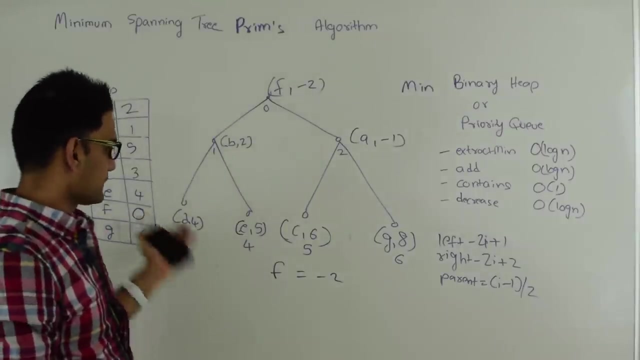 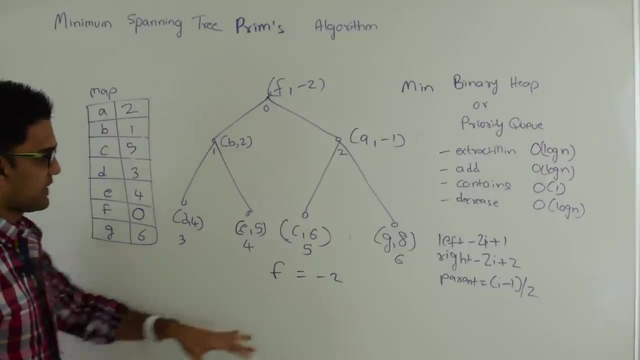 f minus 2 is here. So then now our f's new location is 0 and a's new location is 2.. So this is how we support decreased key operation in ORF log n time. So hopefully this helps you understand how we are going to use these two data structures. 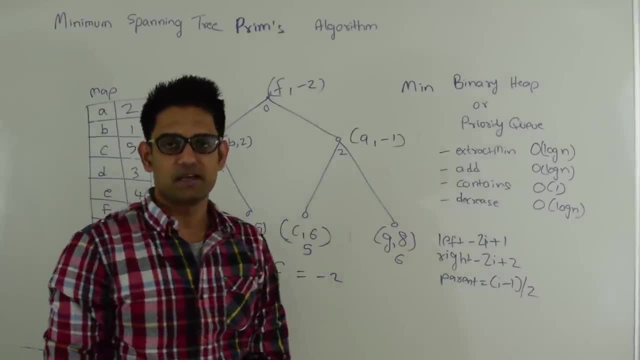 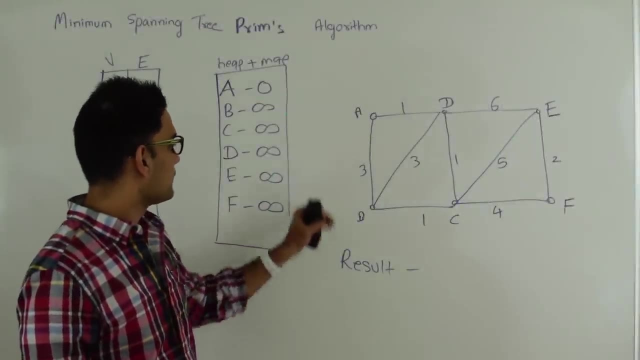 combined together to have these four operations in the prims algorithm. So in the next section let's look at the prims algorithm. The way this algorithm works is: first, we take all the vertices put in this heap plus map data structure which we just discussed with. 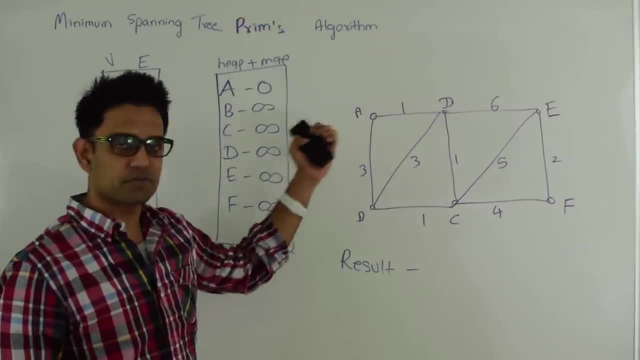 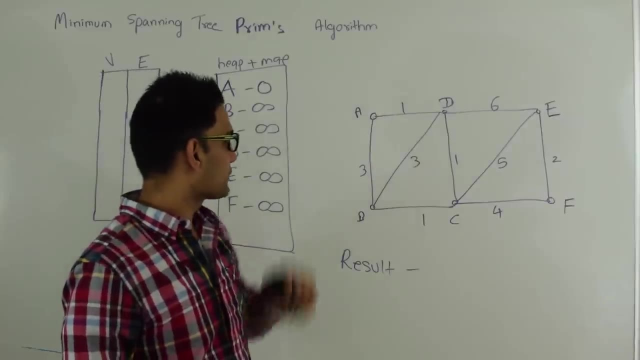 the value infinity, and the node, the vertex from which we are going to start, as a value 0. In this case we are going to start from A, but we can start from any vertex. Then we are going to explore neighbors of A, in this case D and B, and check if the 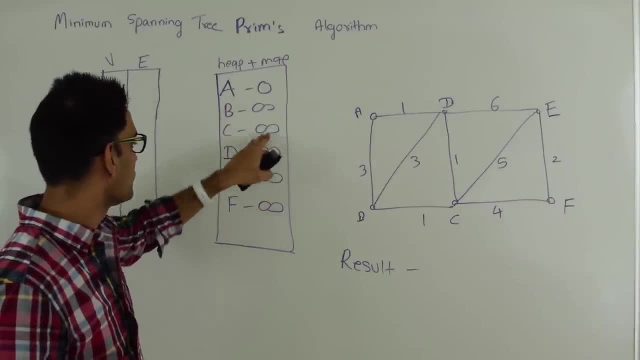 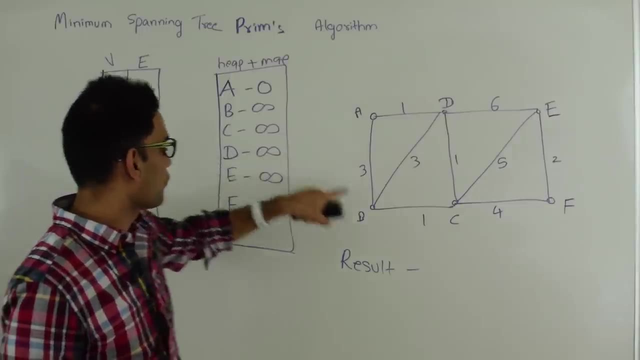 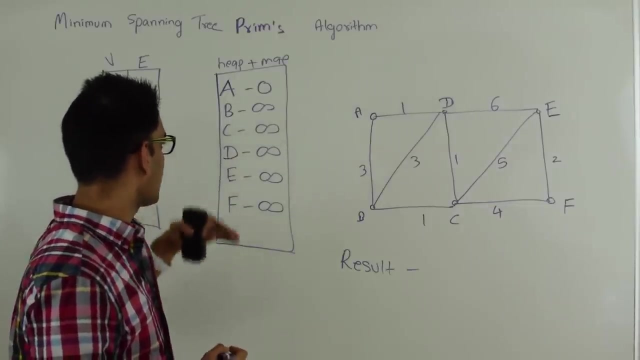 vertices in this heap plus map, and if they do, and if the value they are attached to is greater than this edge weight, then we update their values. So D, infinity, so we update it to 1.. A's value is 3, so we update it to 3, and then we keep repeating this process, then extract. 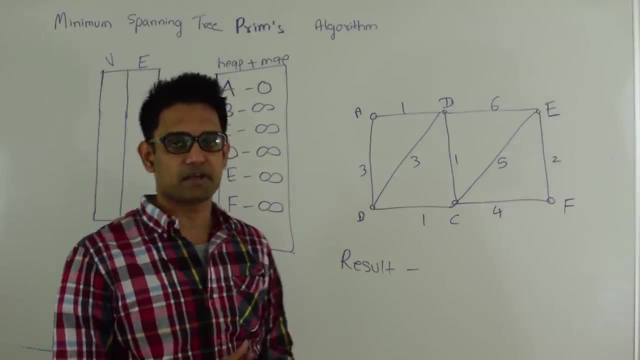 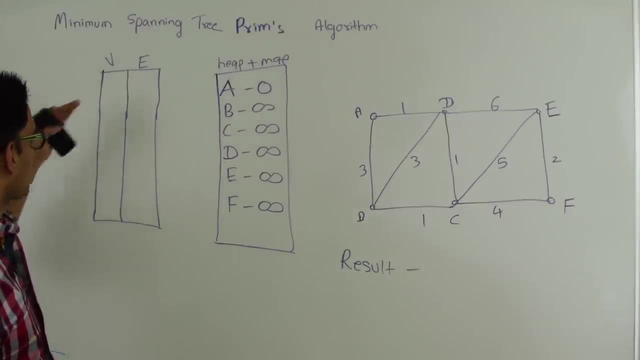 min again and keep repeating this process until there are elements in this heap plus map data structure. Also, we are going to store, we are going to have another map going from vertex to edge which is going to store for, for every vertex, which edge is contributing to the minimum value in this. 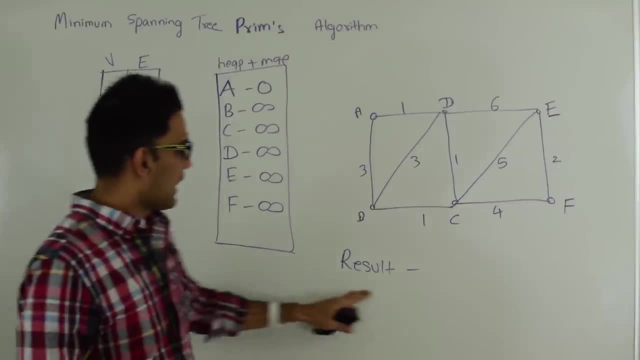 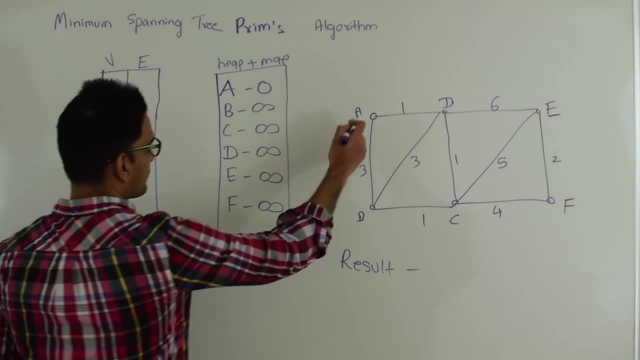 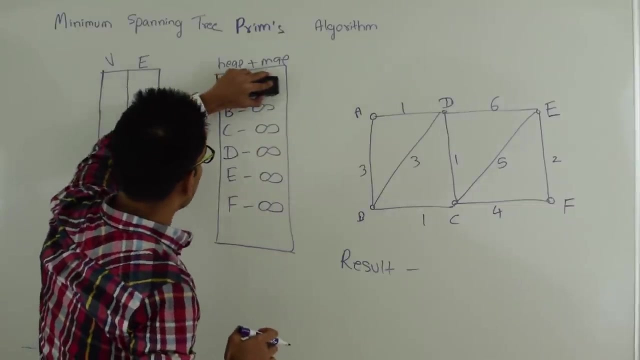 heap plus map data structure. This is to get the final result, and in here we are going to store the final result. So let's do a dry rank on this graph here. So we start from A, we do an extract, we do an extract min here. So the minimum value is 0, so A, So A comes out of this. 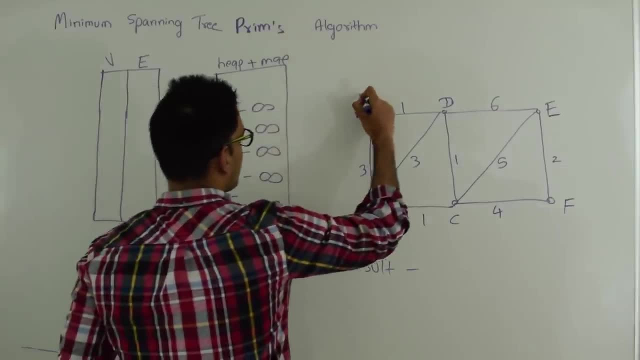 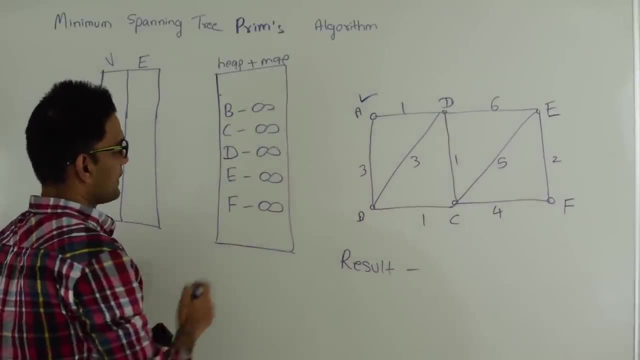 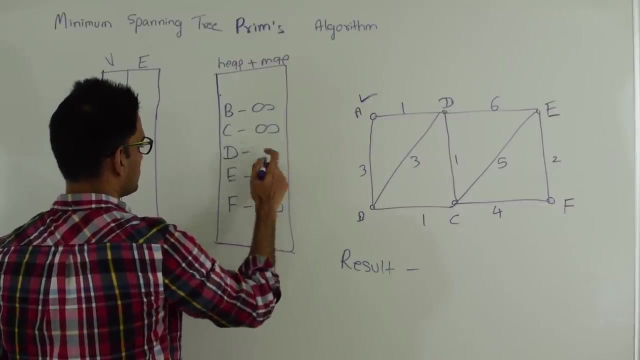 heap plus map data structure. Then we are going to explore neighbors of A. So first neighbor of A is, say, D. So D contains in this heap plus map and the value attached with D is infinity, which is greater than 1, so we update this new value to one and in 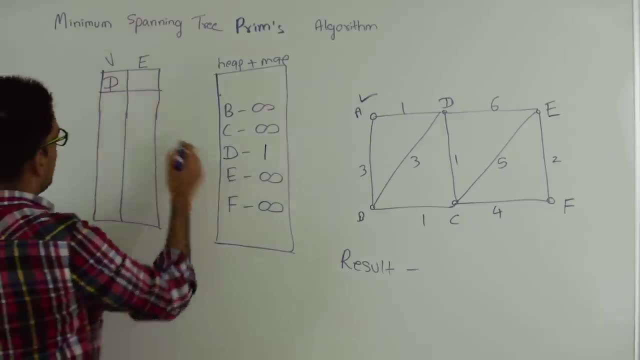 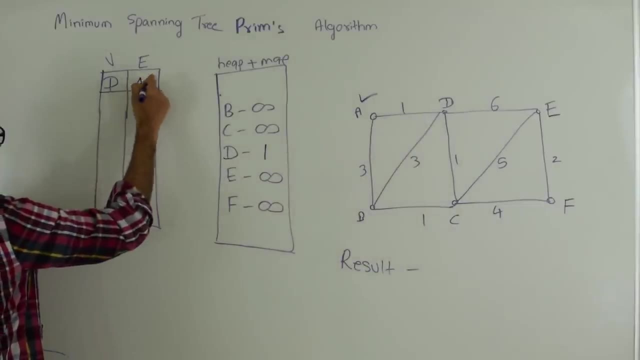 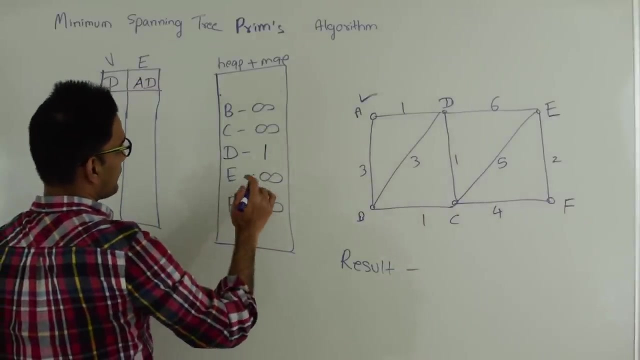 here we are going to store this. Say that D is introduced, the minimum value for D is coming from this edge, AD. Then we are going to explore other neighbor of A, which is B. B is is in this map here and bthe minimum value of b isthe value attached with b is. 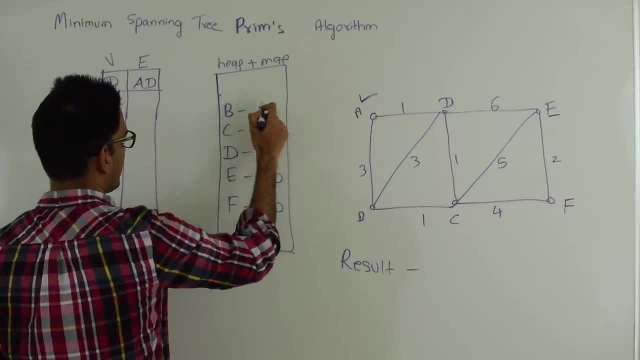 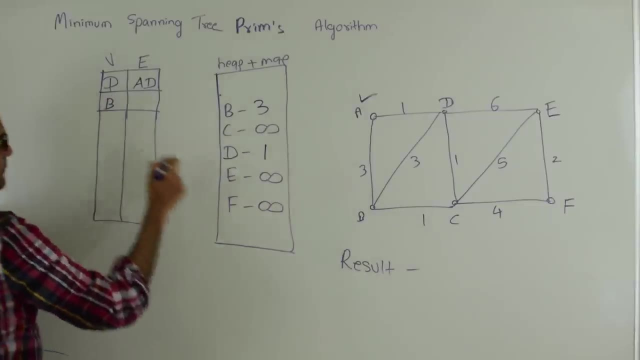 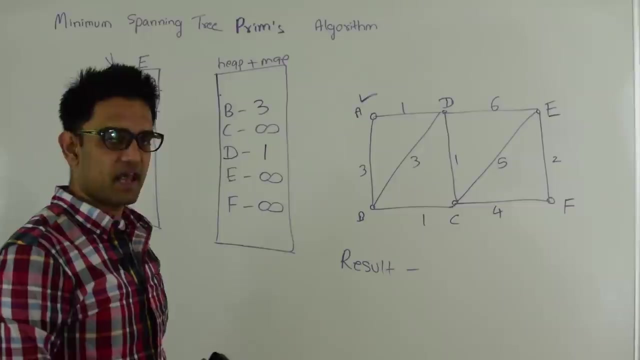 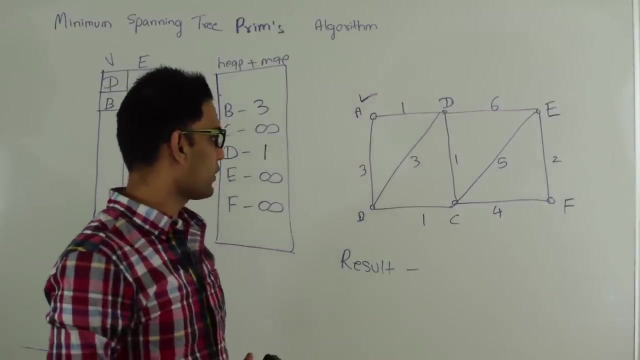 infinity which is greater than 3, so this value becomes 3 and we'll indicate here that b isb's minimum value edge is coming from this edge, abSo, as we discussed heap plus map, the decrease operation can happen in O time and contains operation can happen in off one timeSo at this point we're done exploring all the 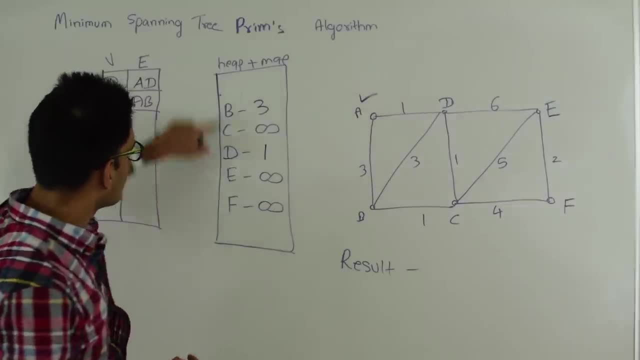 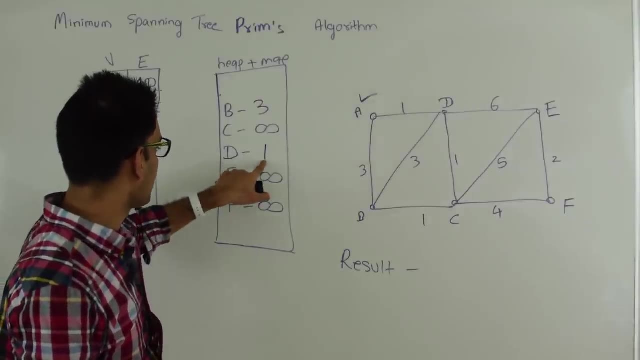 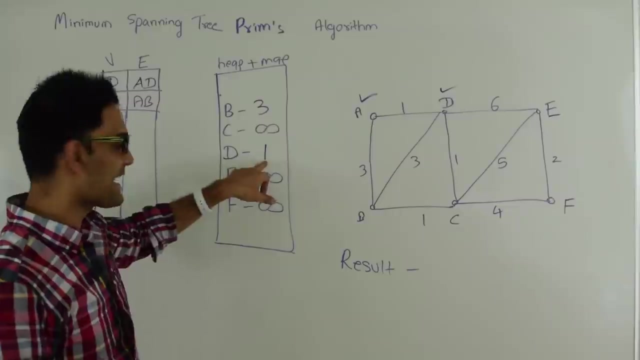 neighbors of a. so we're done with a and then we're going to do an extract min on this heap plus map, which can again be done in off log in time and get the next value. so the next min here is 1.So we'll take 1 out and then we're going to check which edge. 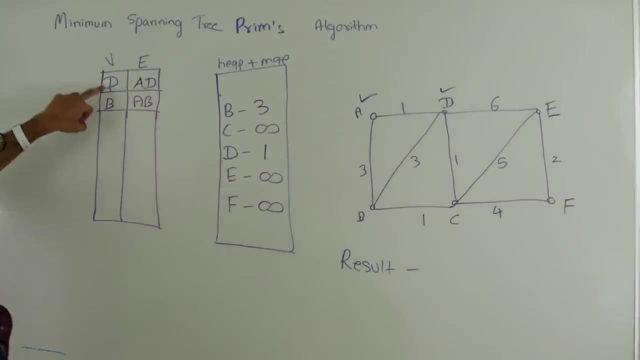 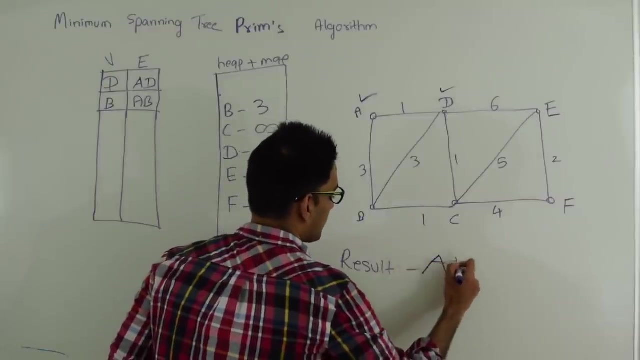 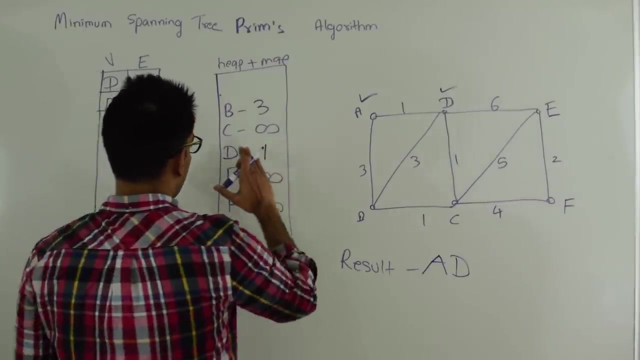 contributed to this value 1, and to do that, we come here and see wherewhich edge contributed to that. So d is ab. edgeSo ab will go into this final result, which has all the edges in the minimum spanning treeThen we're going to remove this guy from here, from this heap plus map. 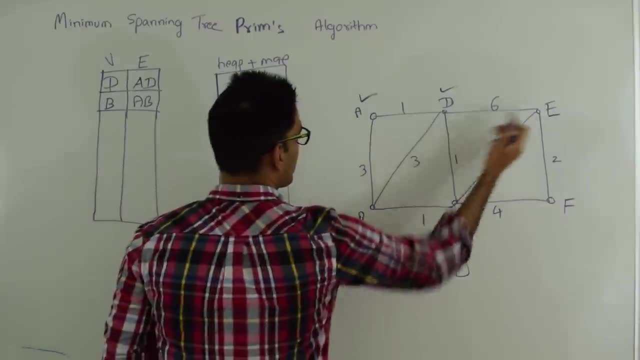 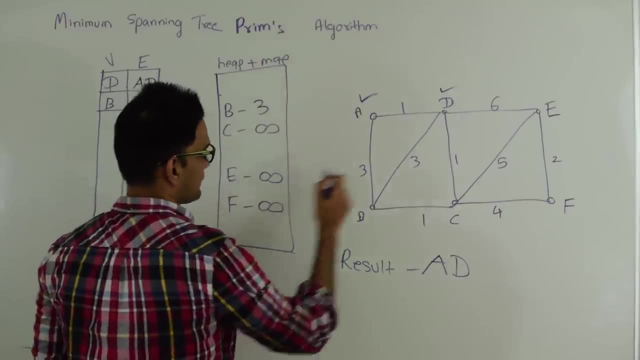 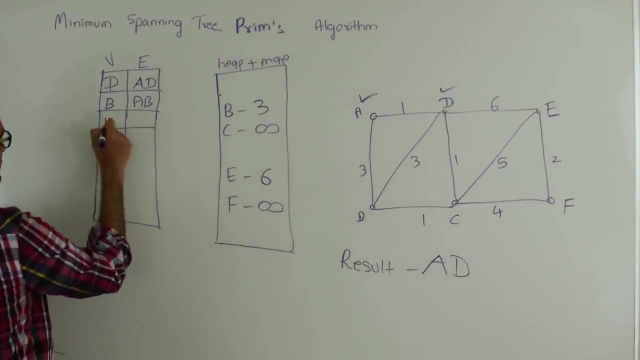 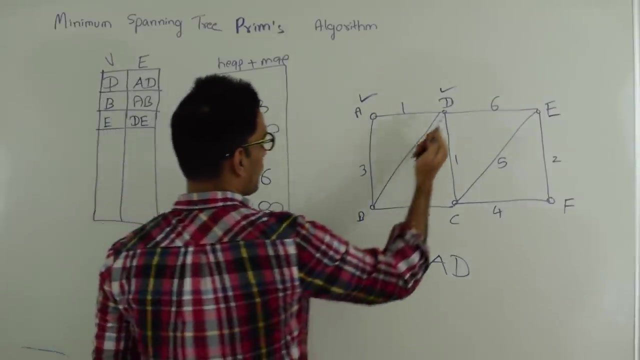 data structure and explore its neighborsSo d's first neighbor is 6 and e is in this heap plus map data structure. it is, and the value attached with this guy is greater than 6, so we'll replace this with 6.. And we will say that e is coming from dThen you'll be. 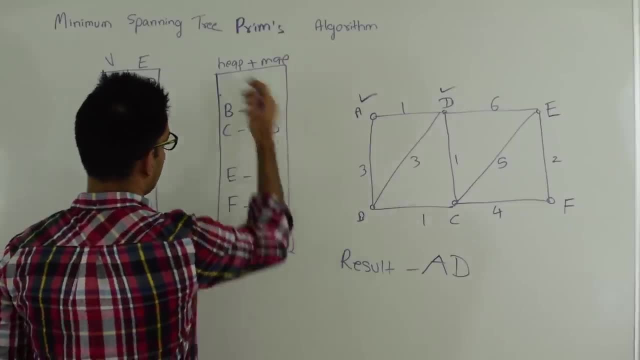 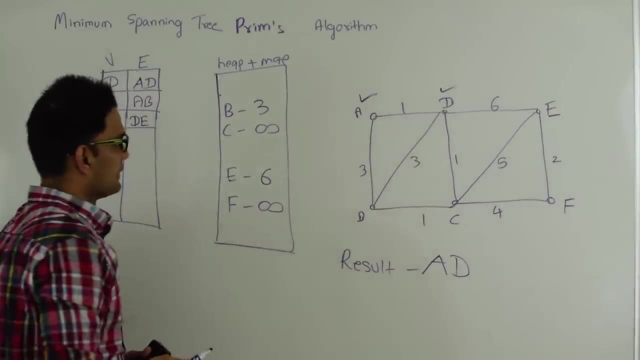 Then we will explore another neighbor of d, so that's b, and the value b is in this heap plus map, and the value b in 3 is not less than this value 3. so we are just going to ignore this edge here. and then you Google, look at the. 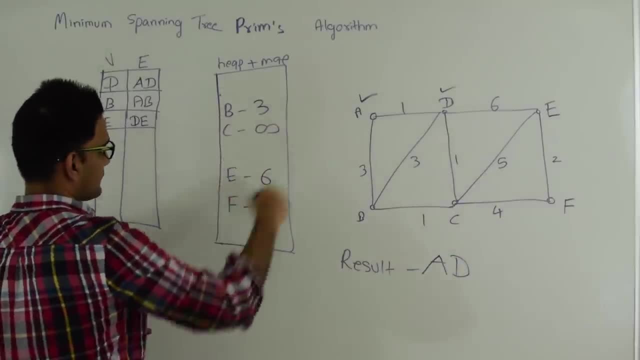 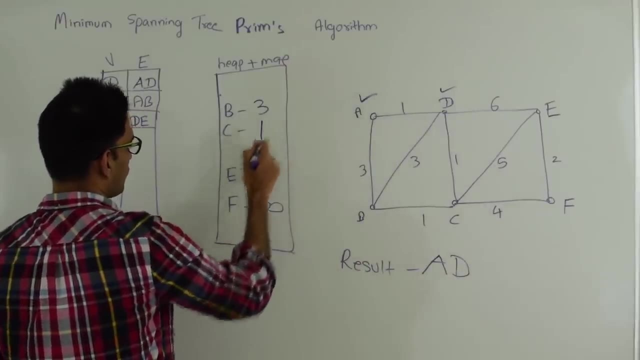 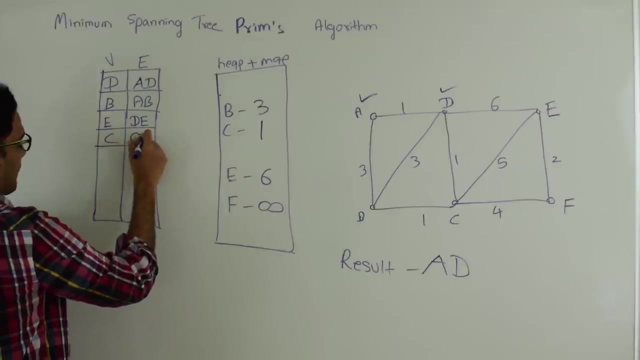 next neighbor of d, which is C. so c is in this heap plus map and the value at c is infinity, which is greater than 1. so we'll change this value to 1 and we'll say that c is coming from dc, cd, hcd. At this point, d is done. 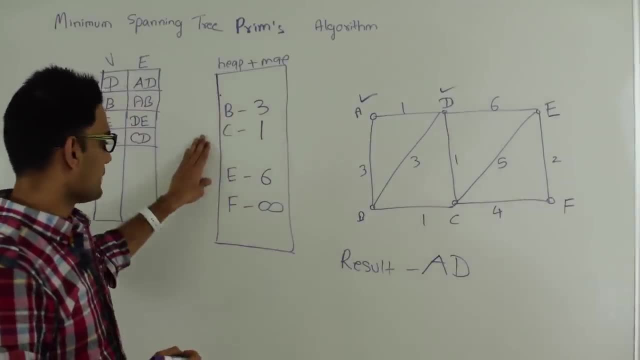 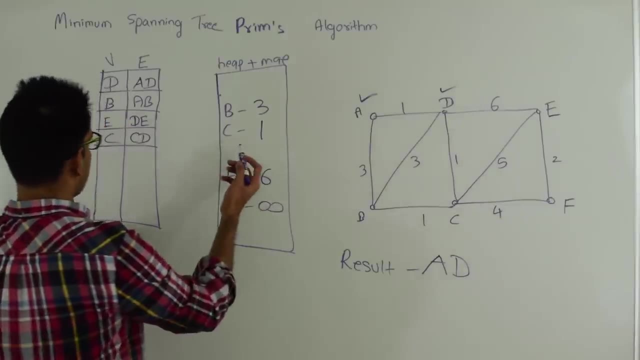 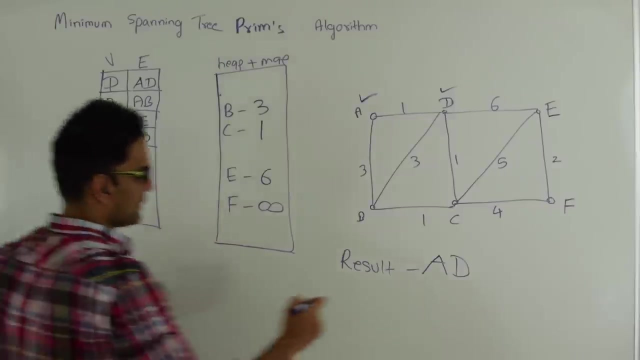 exploring all its neighbors. so we again go into this heap plus map and do an extract min here. So this time c1 comes out. So first thing we check is where who introduced this c1 into this heap plus map, and that's, we go to this vertex and that is cd. So cd. 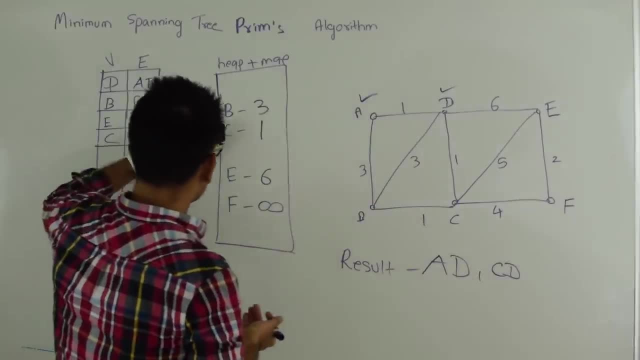 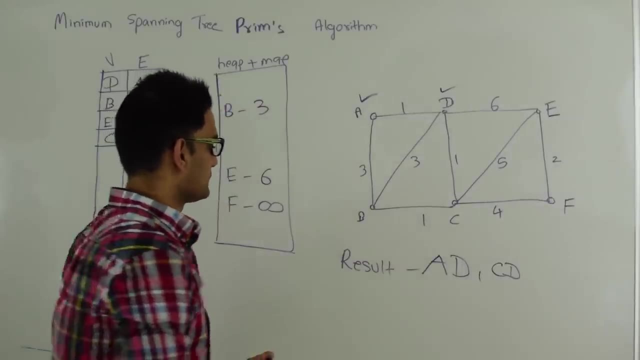 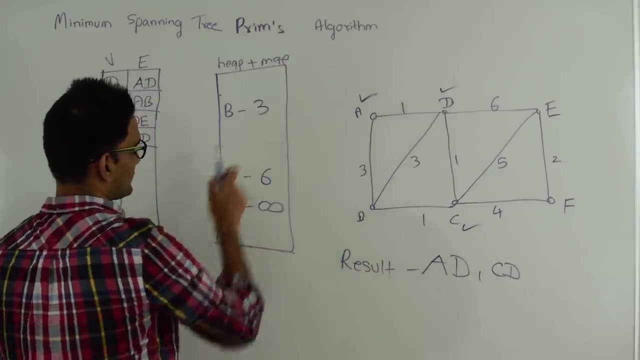 is also in final result and we're going to do an extract min on this heap plus map. Now we're going to explore neighbors of c. So c first neighbor we explore is b. Now the value stored with b right now is 3, while this edge has a weight 1, which is less than 3, so this edge is better. 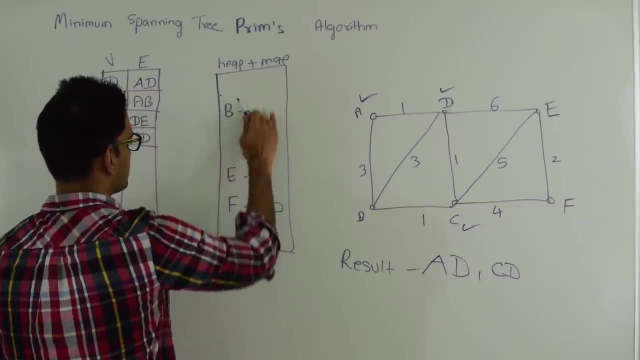 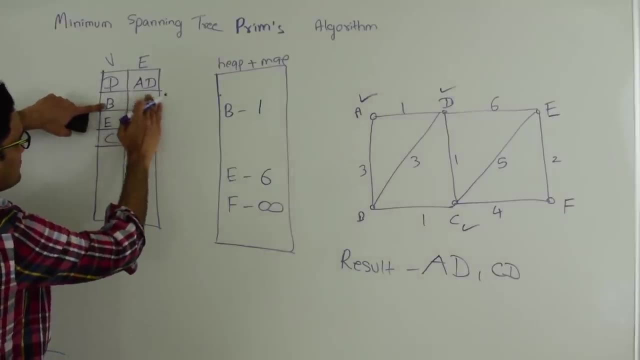 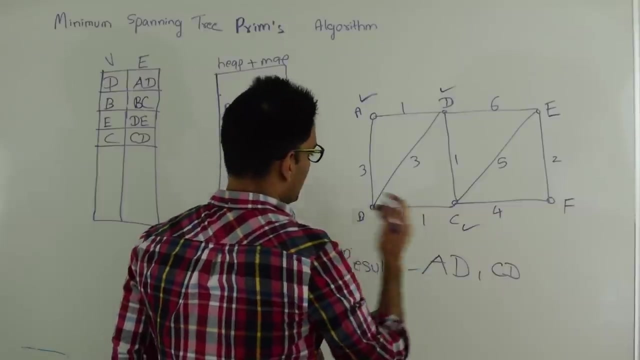 than what we have in here. so we'll change this to 1. And we'll say that b's edge is bc. Then we're going to explore other neighbor of c, So that's d. d is not in this heap plus map data structure, so we'll ignore d. 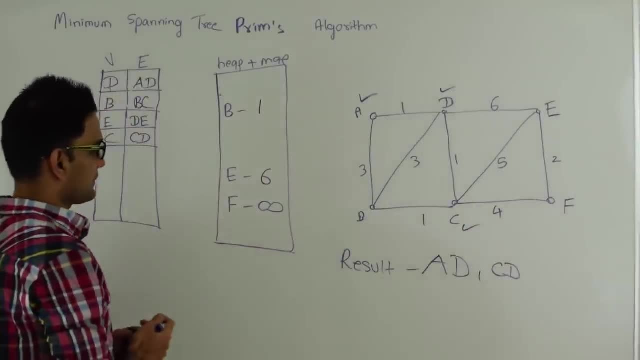 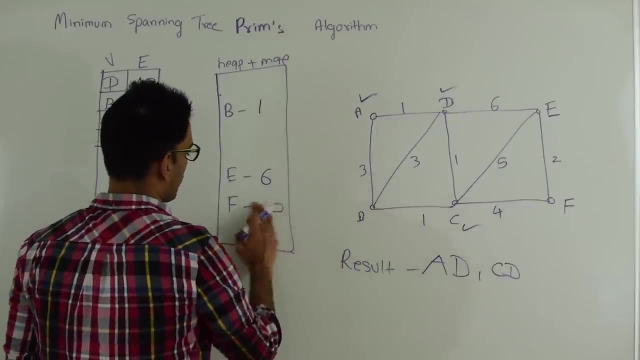 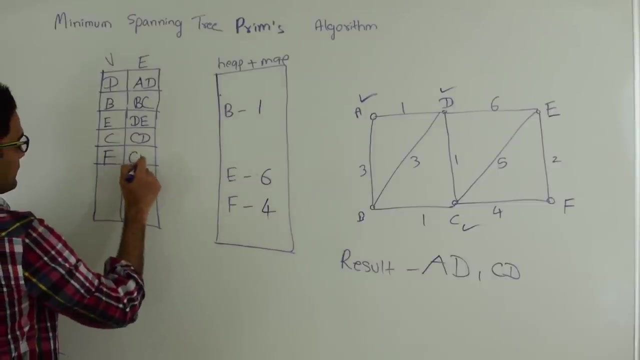 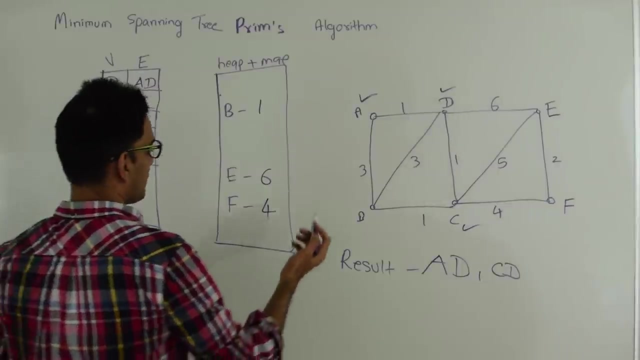 And we're going to explore f. f is there in this data structure and the value attached with f is infinity, which is greater than 4. so we're going to replace this with 4 and we're going to say that f is coming from this edge cf. Then we're going to explore this neighbor e, and the value attached with e right now is 6. 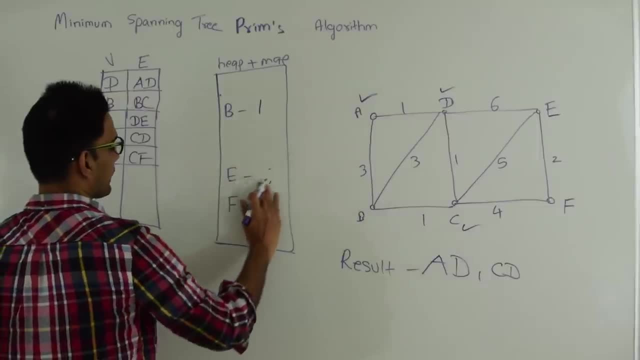 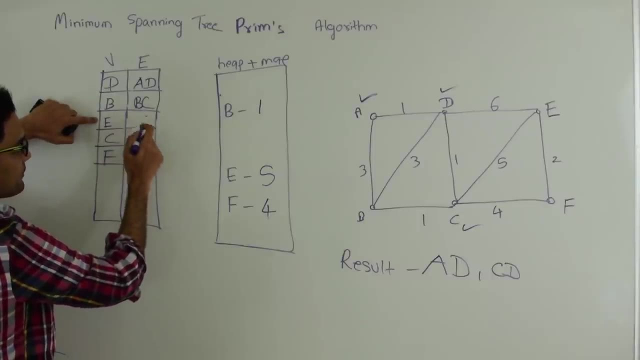 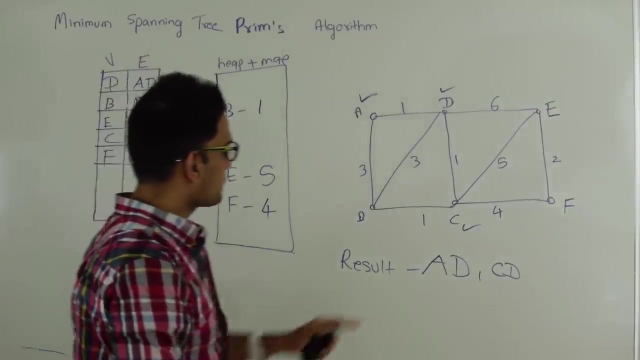 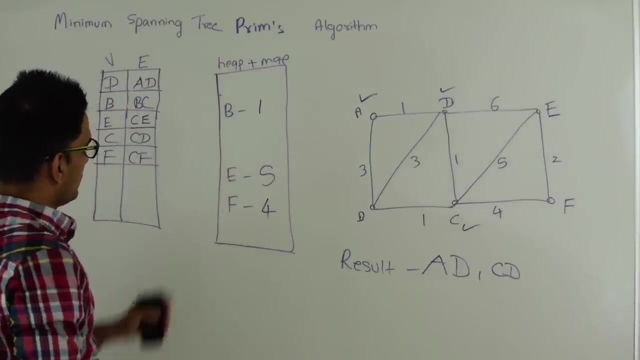 which is greater than this edge weight: 5. so we're going to replace this with 5 and in here we're going to say that e is coming from ce. now, At this point of time, we're done exploring all the neighbors of c, so we again go here and do an extract min. So at this point we're going to extract b out of this. 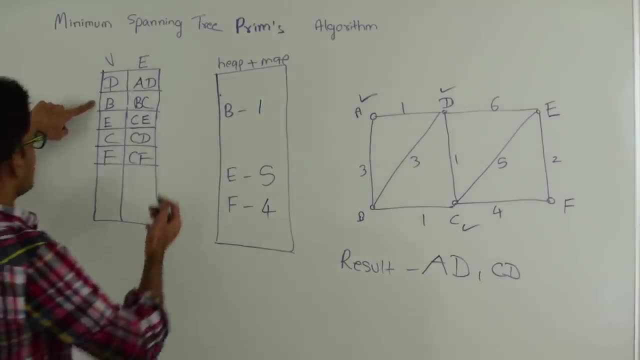 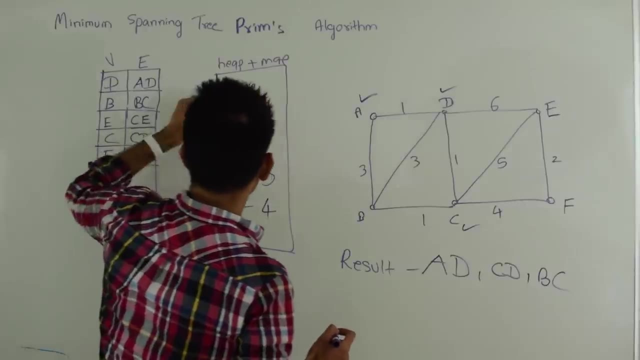 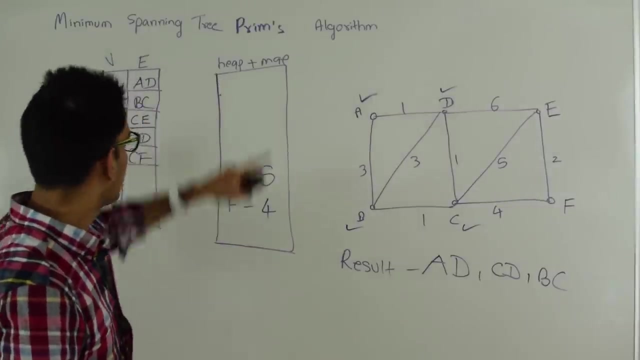 heap-less Mach and we're going to go. and which edge introduced? B and that is BC. So BC will go into the final result and we're going to remove B from this heap plus map data structure. Now we're going to explore neighbors of B. So first neighbor of B is A. It is not there in this heap plus map. 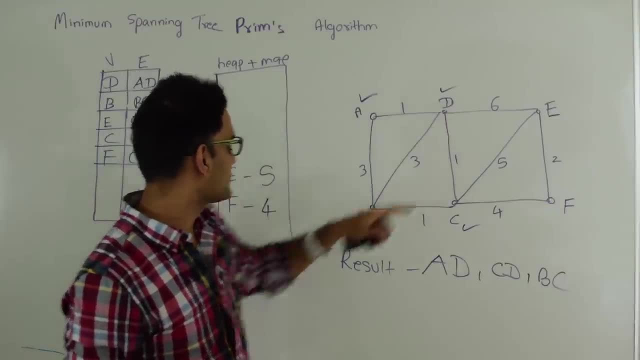 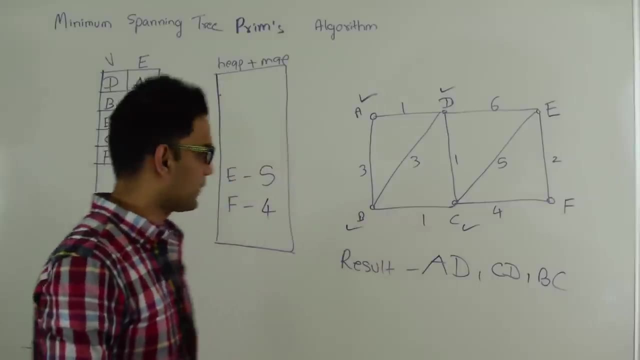 data structure, so we ignore it. This another neighbor is D. D is also not there, so we ignore it. Another neighbor is C. C is also not there in this heap plus map, so we ignore it as well. So now we move to the next. we do again, do an extract, main on this heap plus. 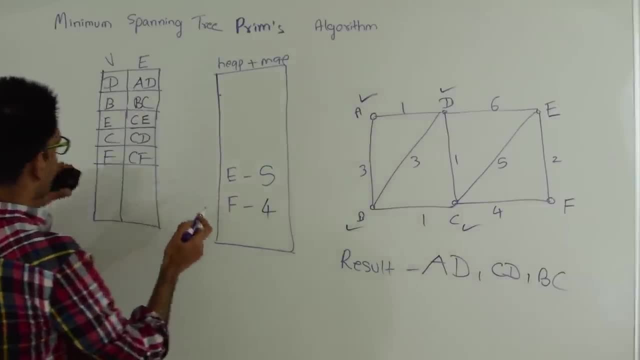 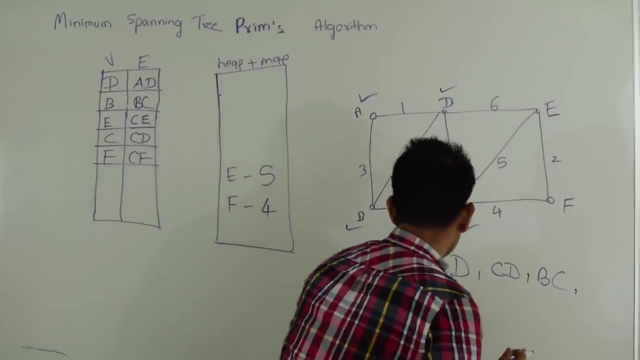 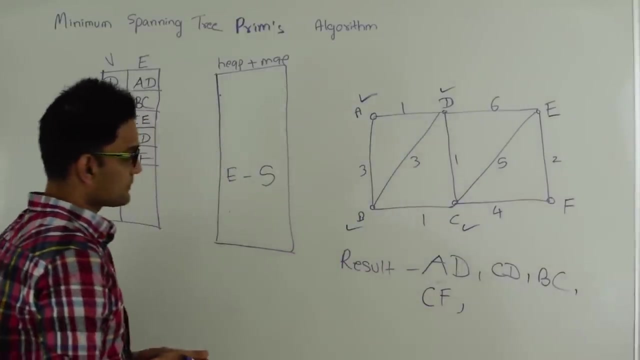 map. So next time we get is: F is 4.. So first thing we do is check who introduced F, and that is edge CF. So CF is also in final result and we'll remove F4 from here. So we'll explore neighbors of F. 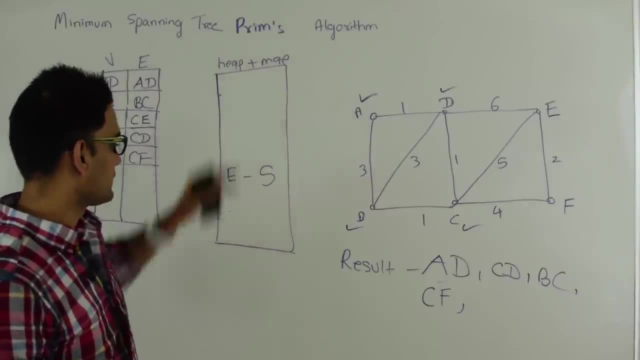 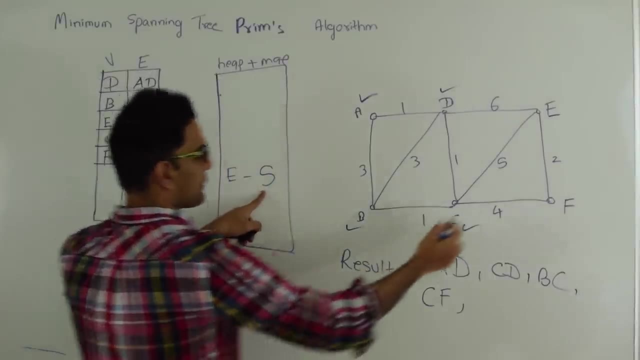 So the first neighbor of F is C, but C is not in this data structure, so we will ignore it. and the next neighbor of f is e, and the value attached with e here is 5, while this edge gets it done in 2, so we will replace this. 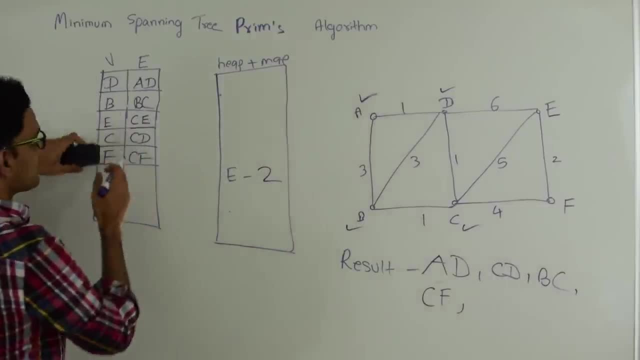 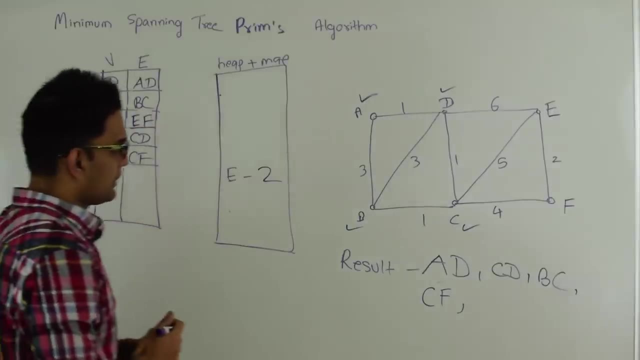 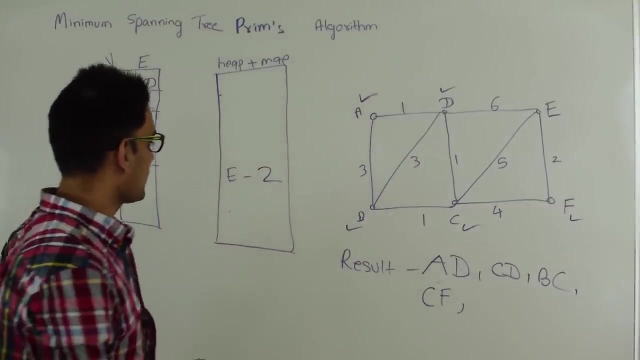 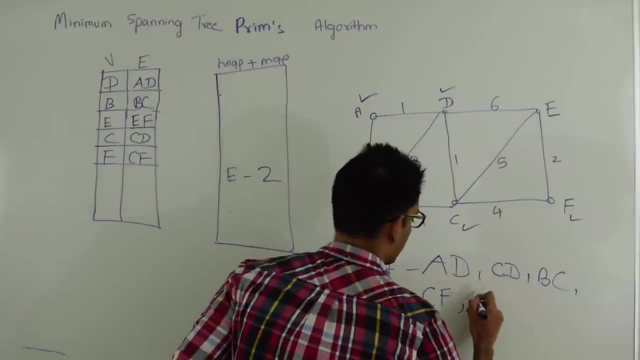 5 with 2 and we will say that e is now coming from ef. and then at this point of time we are done exploring all the neighbors of f. so we go back here and we extract this last guy out and we check who introduced this value to. so that's ef. so ef is also in final result. 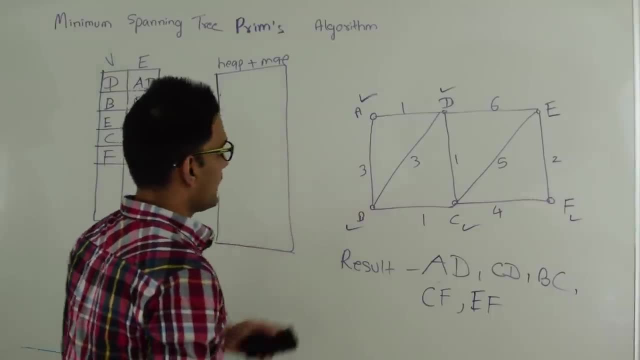 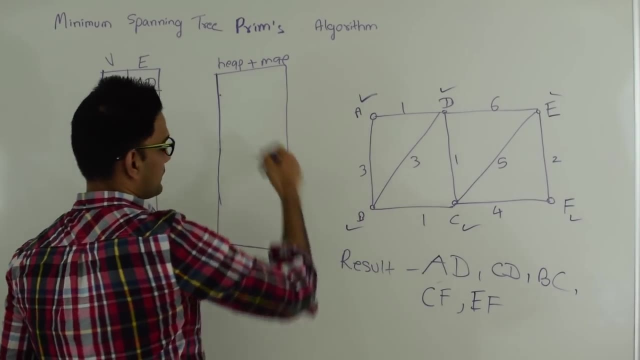 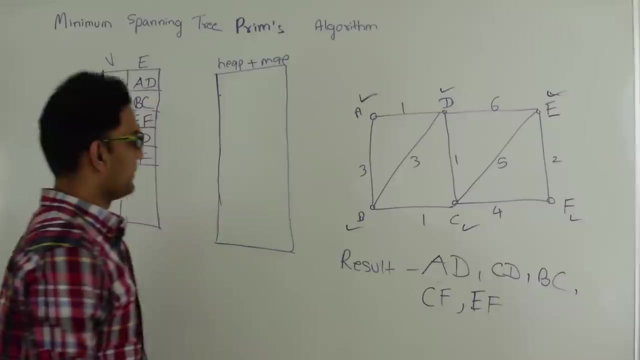 and we remove this guy from here and we will look at it's neighbors. so we go to D. D doesn't exist in this data section, c doesn't existence here and F doesn't exist here. so we are totally done exploring e at this point of time. so we go back here at this point. so this sparkle. 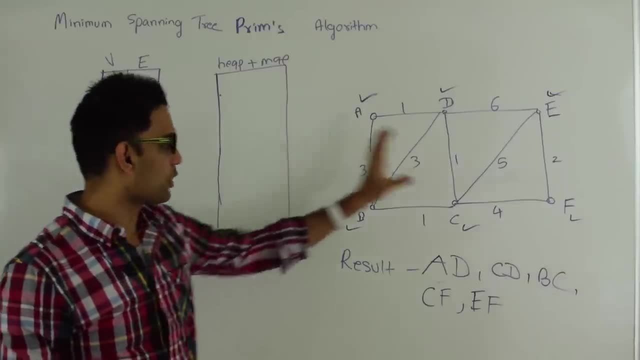 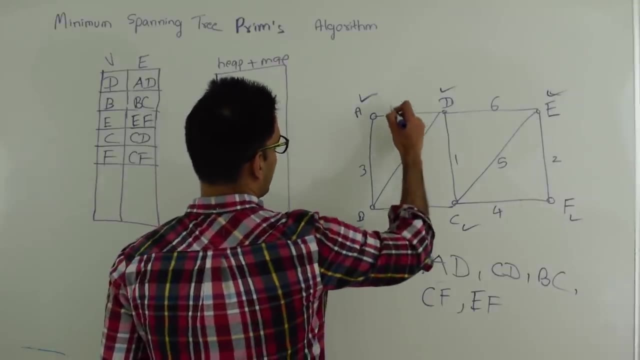 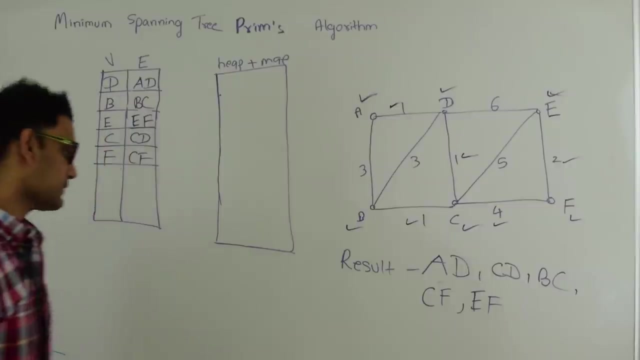 microc bend variable has no elements. it means that all the vertices have been covered and we got our minimum spanning tree edges. So the edges for this minimum spanning tree is this one, this one, this one, this four and this two. So let's analyze the time and space complexity. 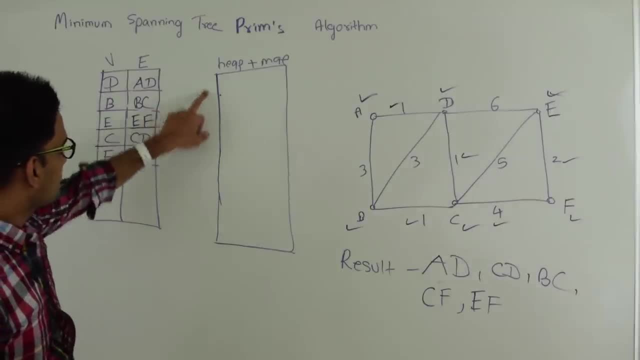 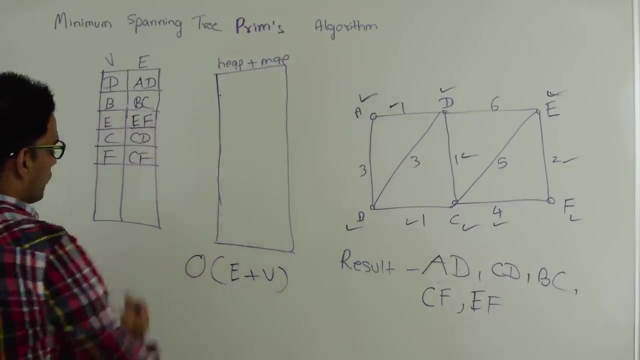 Space complexity is pretty straight forward. This we are storing. result: we are storing this map and we are storing heap plus map data structure. In the worst case, the space complexity will be e plus v, because we might have to store all the edges of this. 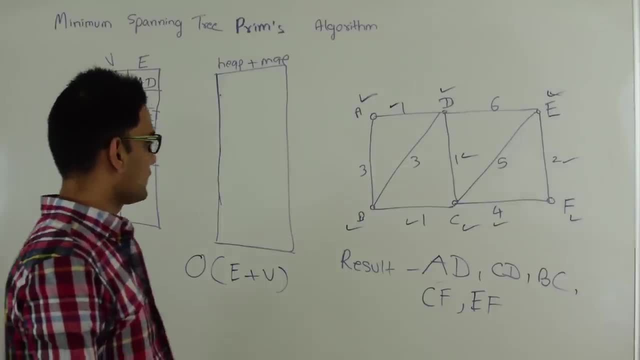 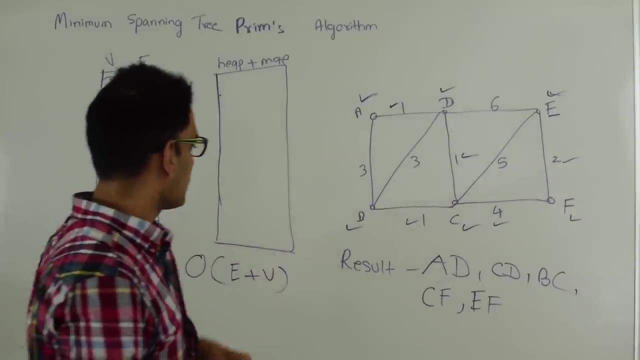 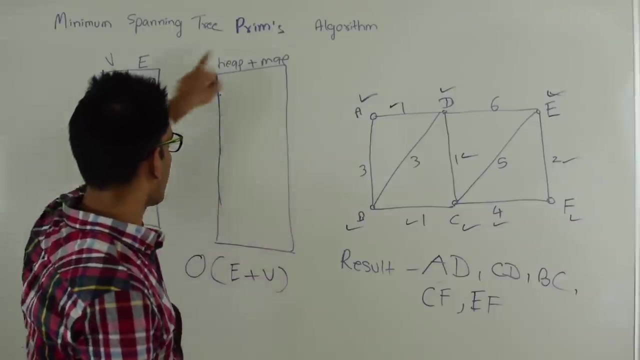 graph. What about the time complexity? So we are performing this operation on. so we are performing so as many edges we have. we are performing that operation that many times on this heap plus map data structure. In the worst case, the size of this heap plus map data structure will be o of v. 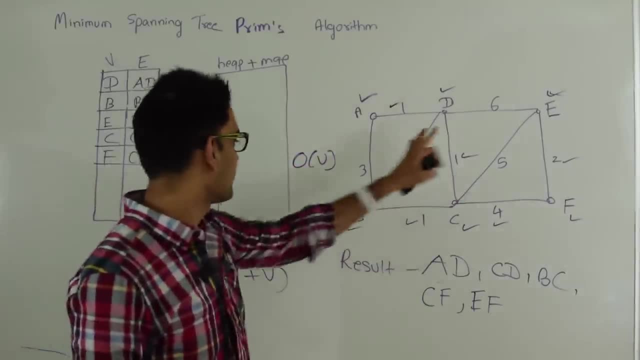 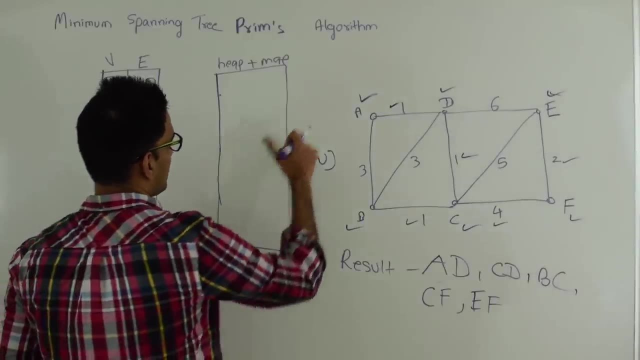 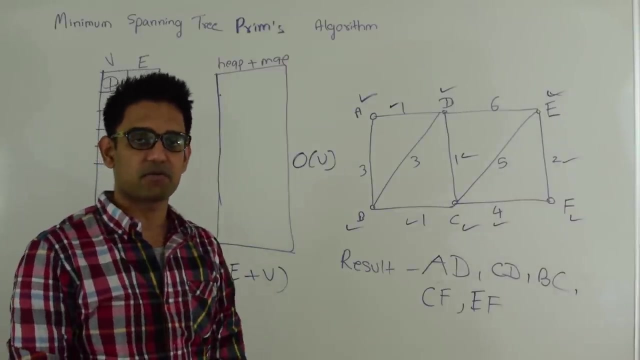 Basically the size of the entire heap, entire graph, And we are doing, in worst case, E operations on this thing and we know that contains works in o of 1 time, extractmin works in o of log n time and works in o of log n time and Decreeski works in o of log n time. 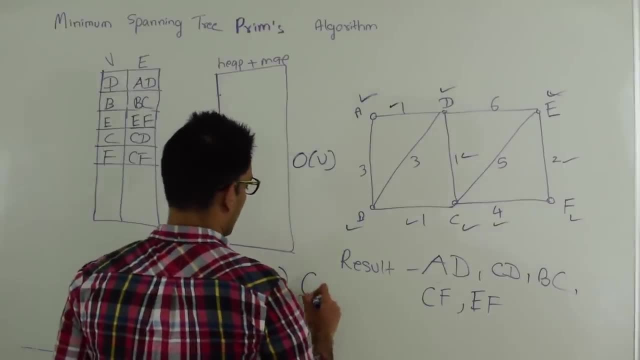 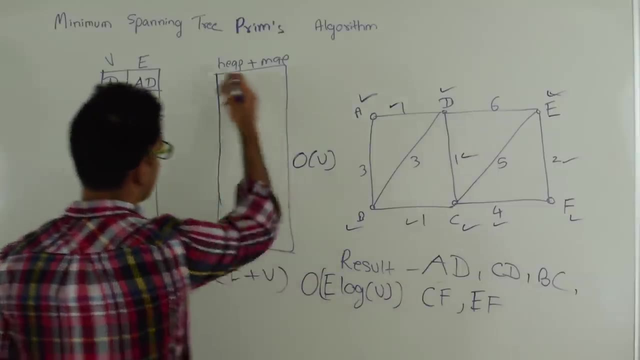 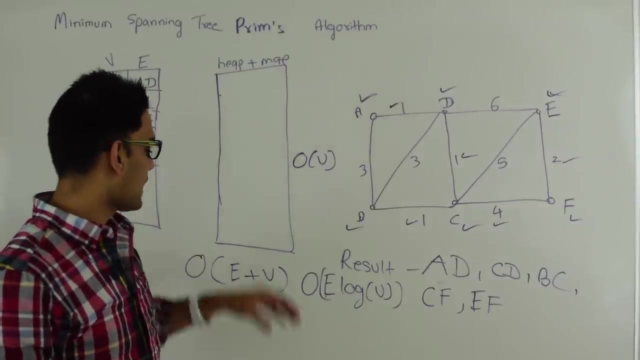 So in worst case the time complexity will be o of E into log of v, where v is the size of this heap plus map data structure. So again the space complexity is O and then the time complexity will be O. So in the next section let's look at the code for this algorithm. 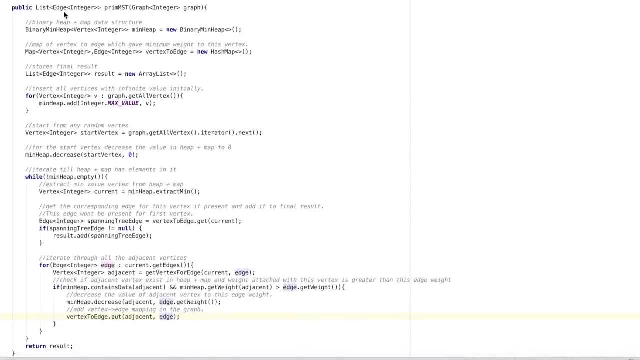 So the name of the function is primmst. It takes in a graph and returns a list of edges which form the minimum spanning tree. Let's first initialize the data structure which we are going to use. So the first one is the binary main heap, which is the heap plus map data structure I discussed in before. 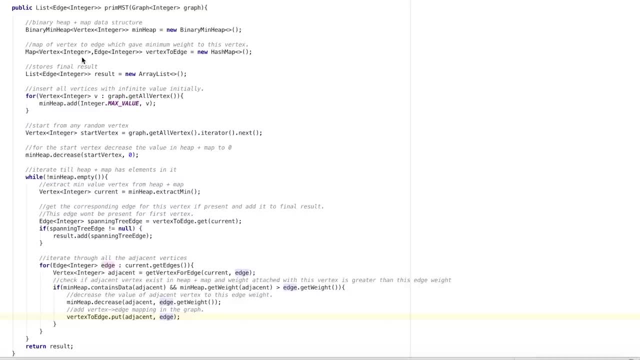 So, if you want, you can look at the class to see how I've implemented it. Then the next data structure is a map from vertex to edge, basically storing the edge which provided the minimum value for this vertex in this main heap. And then, finally, this is a list of edges which is just going to store the final result. 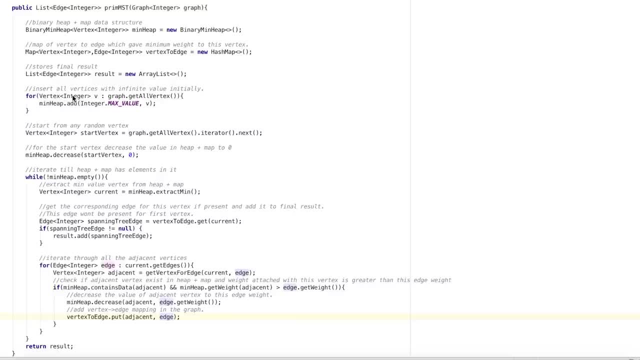 So first thing we do is we iterate through all the vertices In this graph and add them to the main heap with the value integer dot max value, which is basically an infinity value, And then we randomly select a start vertex from this graph And then decrease the weight of that vertex in this main heap to zero. 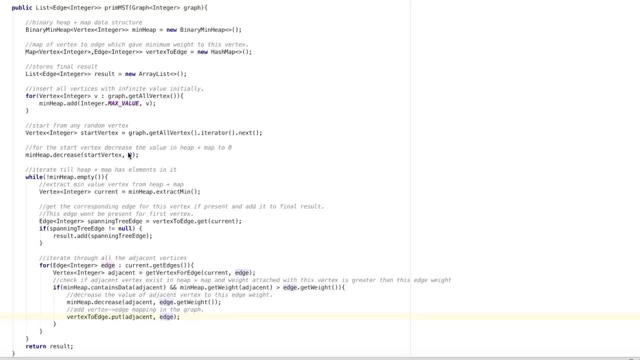 So basically, this is the first vertex which will get selected, And then we go into this while loop until this main heap is not empty. Then we select A vertex, So then our current will be. the first will be the minimum value vertex in the main heap. 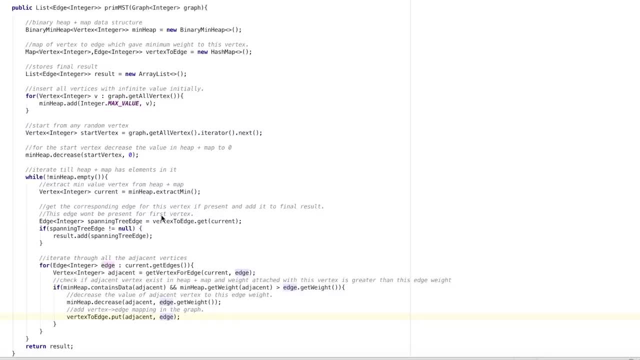 And then we check if this current has a corresponding edge in this vertex to edge graph map or not. So this will be missing for the start vertex, but this value should be available for every other vertex. So we check if spanning tree edge is not null. 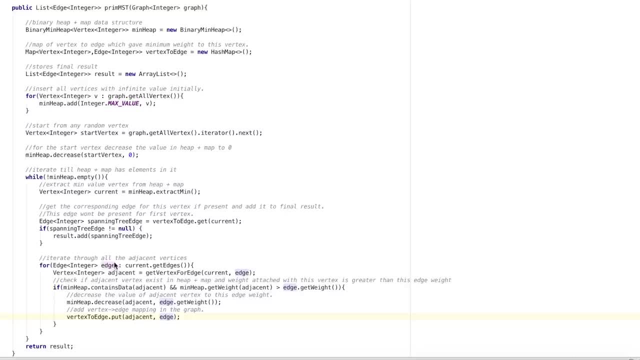 If it is not, then we add it to the final result. Then we are going to get every edge for this current vertex And then get the adjacent vertex for this edge And then we are going to check if this adjacent vertex exists in the main heap or not. 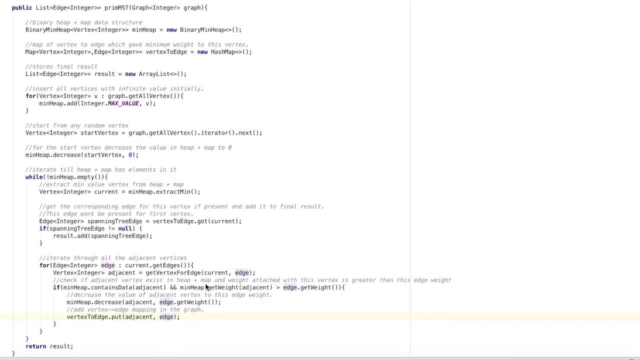 And if it does exist, then is the weight attached with this vertex is greater than the edge weight or not? If both the conditions are true, basically if it exists in the main heap And the weight attached, the current weight attached with this adjacent vertex, is greater than the edge weight, 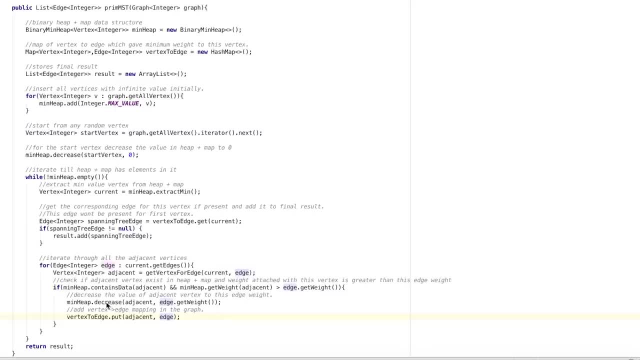 Then we are going to go into the main heap and decrease the value of that vertex to the current edge weight And then we are going to add this vertex and the edge into this vertex to edge map And then we are going to repeat the process for other edges of this current vertex. 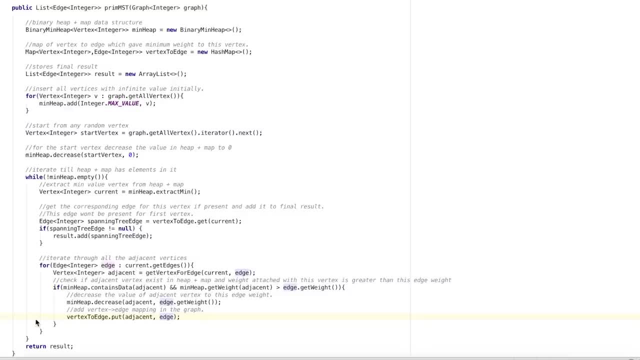 And once we are done totally exploring this vertex, We are going to go back and go to the top and repeat the same process, Basically again doing an extract min and getting another current vertex And then going through its neighbors and updating the main heap. 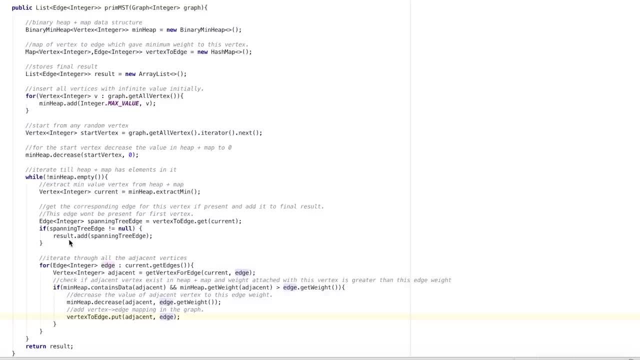 And finally, the final result will be stored in this result list And we will just return this list. So again, the time complexity is O and space Time complexity is E, log V And space complexity is O. So this is all I have to talk about prims algorithm. 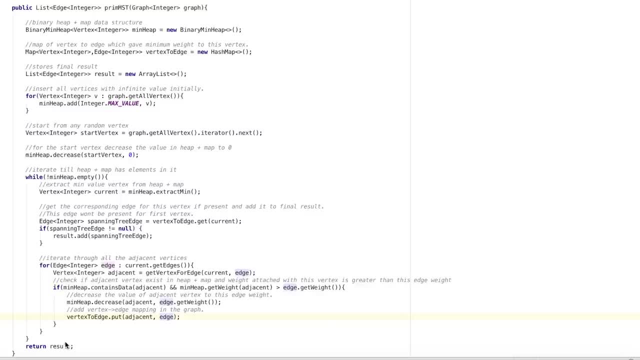 Please like this videoshare this videocomment on this video. Check out my facebook page: facebookcom- tusharoy25.. And check out my github link: githubcom. mission piece interview wiki. Thanks again for watching this. 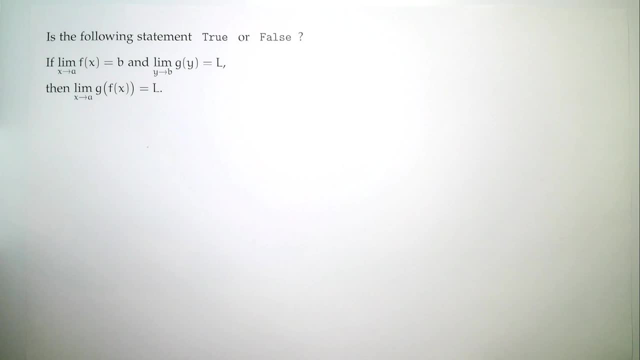 Well, you know, we always like to start with a problem, a nice warm-up problem. and so here we go. a nice warm-up problem. Is the following statement true or false? If the limit as x gets close to a of f of x is b and the limit as y gets close to b of g of